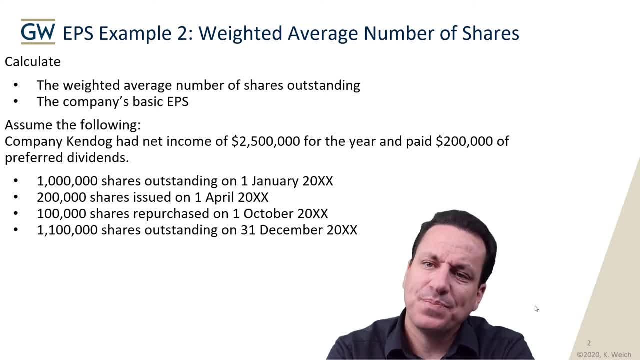 of these shares And what's the weighted average number of these shares? And what's the weighted average number of these shares And what's the weighted average number of these shares? And what we're trying to get at here is that the shareholders are not there for the whole year. 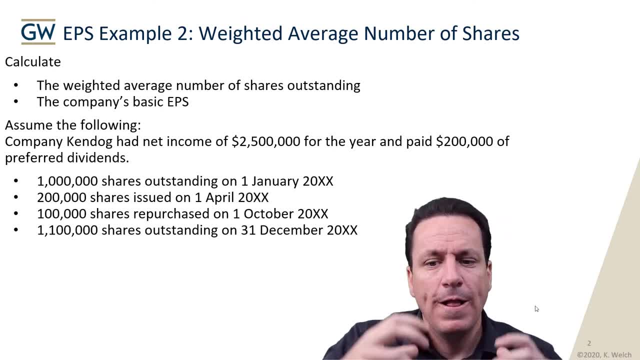 But the earnings, what we use for our earnings per share, is there for the year. When you report net income it's January to December. But you don't want to give January to December. You don't want to give everybody credit for being at the table the whole time if they showed up late to. 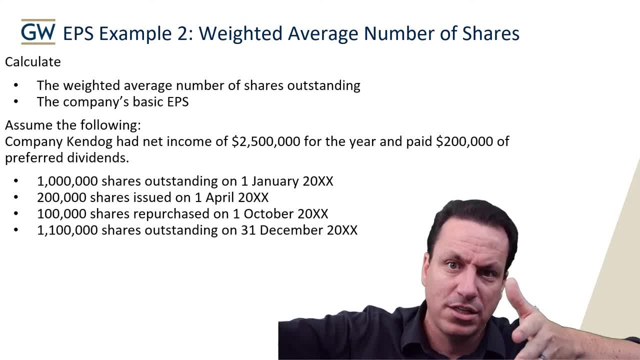 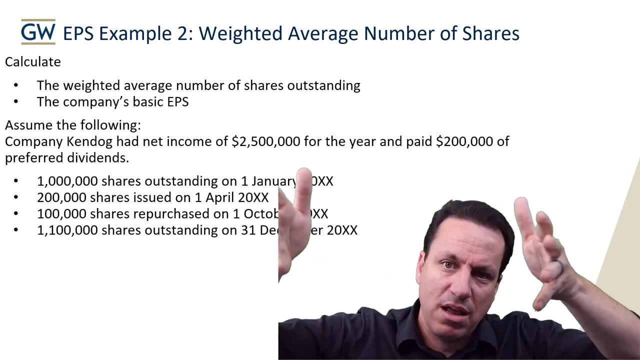 dinner, or if they left early from dinner, They didn't get to execute. They're not there the whole time. So we have to find out what the earnings is going to be for everyone showing up and leaving. and factor that in, We're kind of getting a weighted average of the time that is. 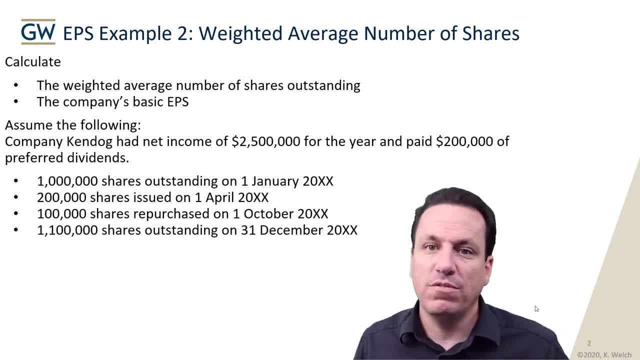 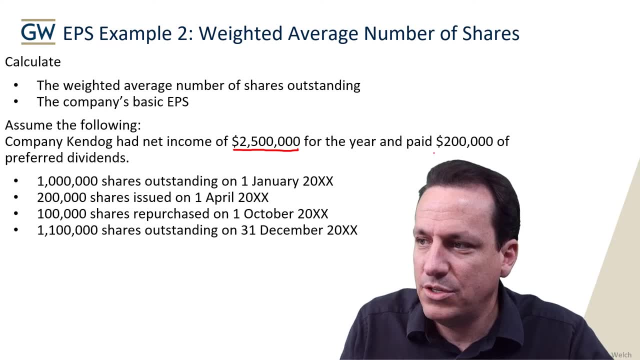 there And we're representing that as the number of shares, the weighted average number of shares outstanding over the entire time period. This right here, this was their net income, And then they paid $200,000 of it in preferred dividends. Pay their preferred dividends, That means common. 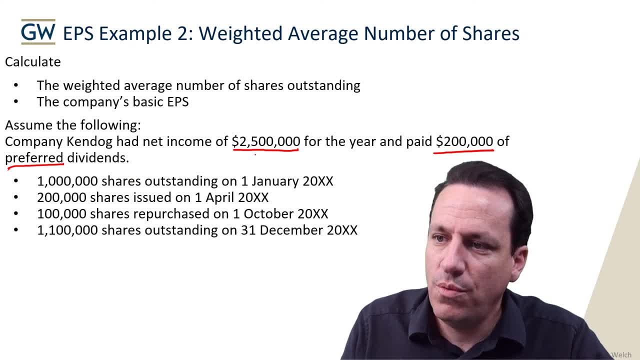 shareholders aren't getting them, We have to net these out. So the $2.5 million gets netted by $200,000 right here. And when we net this by $200,000, we're going to get $2.3.. So that is what's. 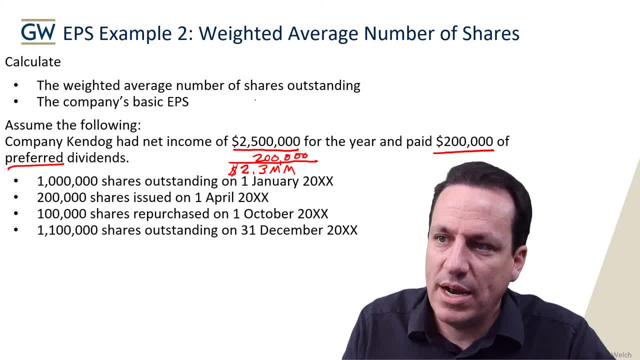 going to go in our numerator, right? So is that the weighted average shares outstanding? No, that's going to help us with our basic EPS. That's going to go in our numerator, All right. So we have 100,000 shares, We have 1 million shares outstanding January 1st And we end up with 1.1 million shares. 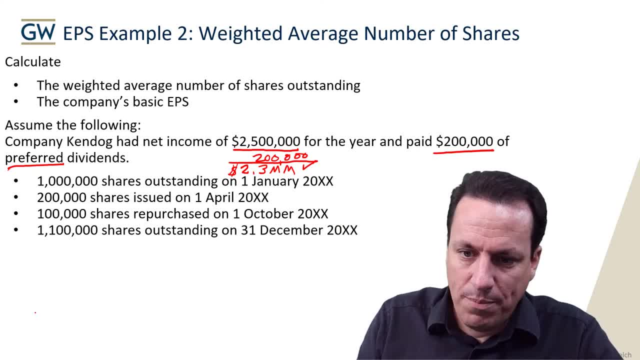 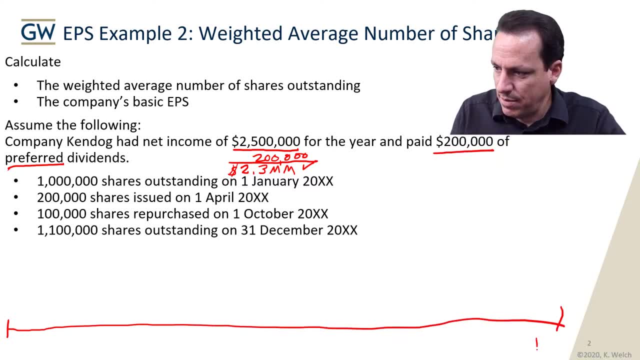 outstanding January, 1st of December, And so what we're doing is- and I'll represent this in kind of like a timeline- Forgive me for my bad writing here, But imagine this is the year and this is December, And this is the 1st of January. Okay, And then we have our different points in the year. 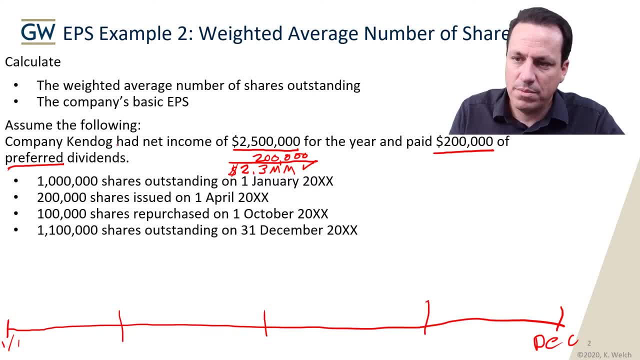 where we have different quarters And the problem's made a little bit easier because this is at the start of Q2.. All right, So for all the way through the three months of January, February, March, three out of 12 months, we have how many outstanding? We have 1 million. 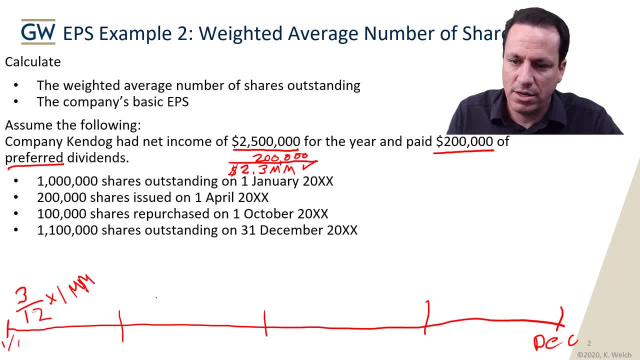 shares outstanding, That's two M's 1 million share outstanding, right. And then what happens? April 1st, April 1st, we have not 1 million, but we have 1.2 million shares outstanding. And how long do we have them outstanding for? All the way from April 1st, all the way through. 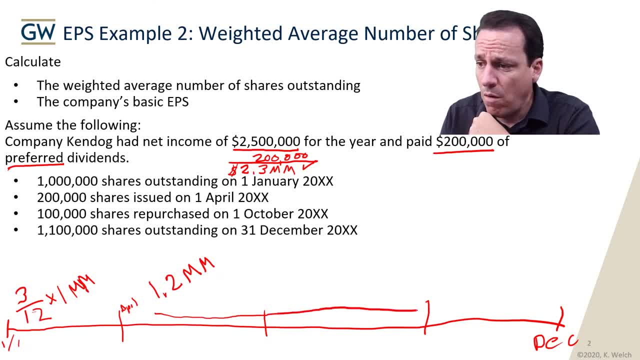 June, July and all the way to October, October 1st. All right, So it's all the way to October 1st. So how long is this 1.2 million outstanding? Well, it's outstanding six out of 12 months. 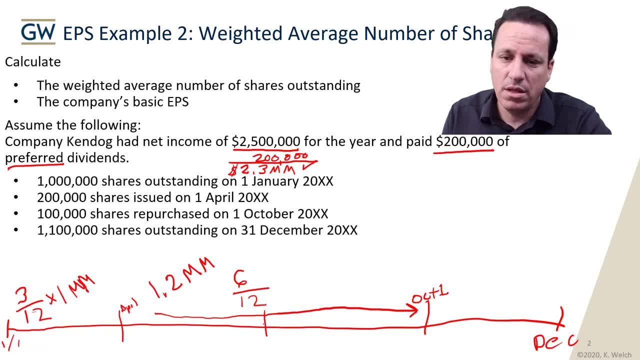 Isn't that so nice that it's like all on even dates. It wasn't on this quarterly date. We just take whatever how many days it is into the year and divide it by three. So it's all on even dates. But because we're dealing with months here, we can use the six months over 12.. So the six over 12,. 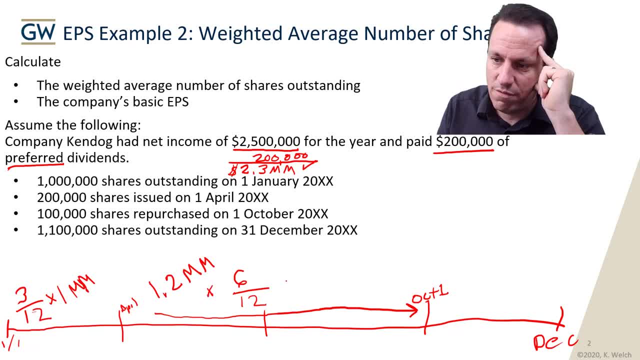 we take the 1.2 million times the six over 12. And that gets us what our weighted average would be for this section of the year. And then at the end of the year we have 1.1 million shares outstanding. times times how many months are left. Three out of 12.. It's always good to just check. You got. 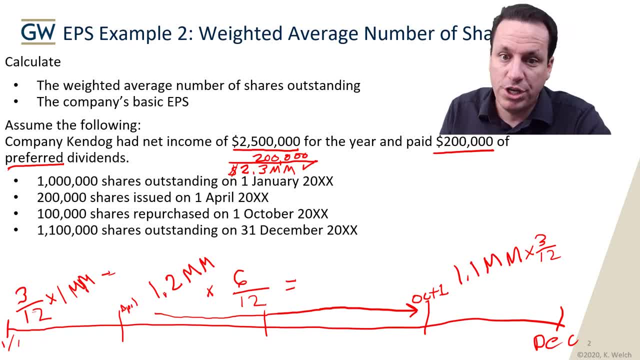 three plus six plus three, It's 12.. So we have a full year's worth of time here, And we have the different time periods where there is a different amount of shares outstanding, And what we're going to do is we're going to take. 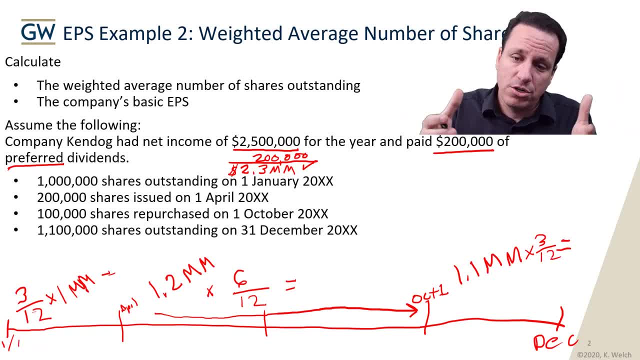 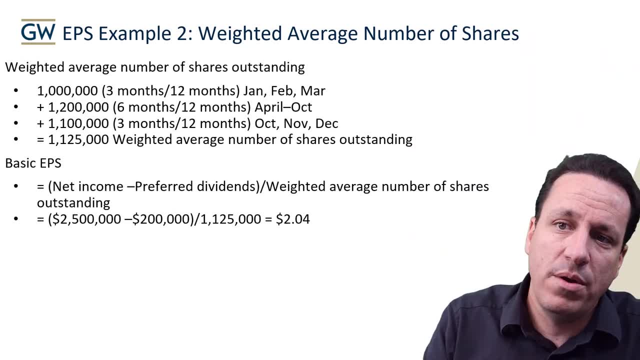 each of these time periods, figure out how many shares of the year they were outstanding for, and then we're going to add them all together, And that's what I've done in this next slide. here We take the 1 million times the three over 12, January, February, March- 1.2 times the six over. 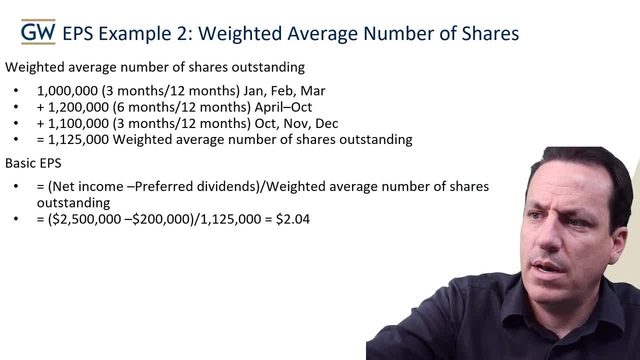 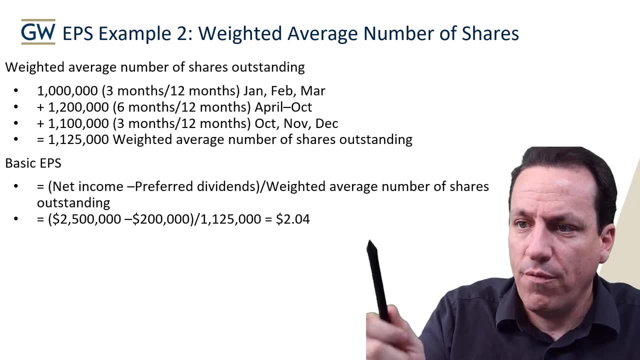 12. And then, and then- and it's important to know that that's the start of October, So it's six months there. And then it's 1.1 for the three months October, November, December. Okay, So, 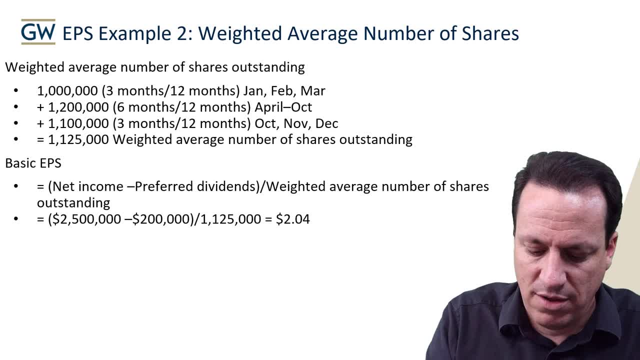 in the total. if you do this, you get a total weighted shares outstanding. If you do this calculation, you get a total weighted average number of shares outstanding here of 1.125 million shares. That's the denominator. That's the denominator in our basic EPS. So when we do